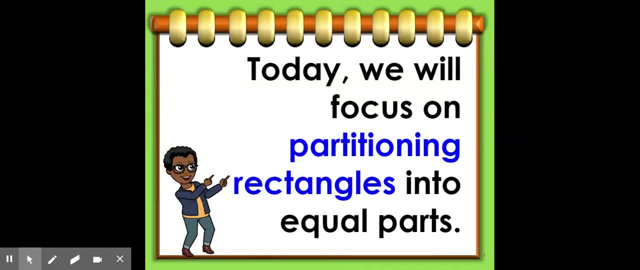 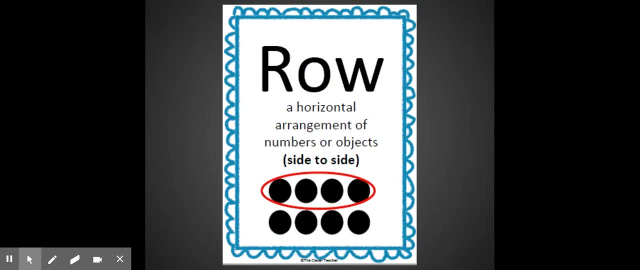 Now that you have finished your time to climb, it's time for us to move on to the second part of our lesson, where we will focus on partitioning rectangles into equal parts. Remember this important vocabulary: A column means that objects are arranged up and down, and a row means the 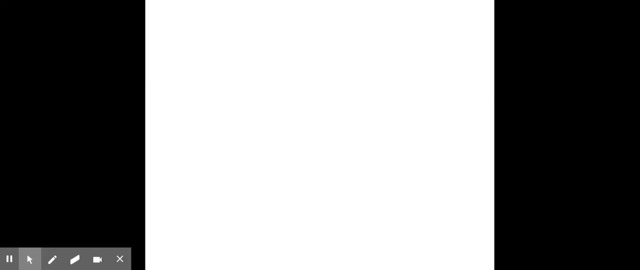 objects are arranged side to side. Let's take a look at this rectangle. We need to partition this into equal rows and equal columns First. we're going to start with the number of rows. It looks like we have one, two, three rows. Let's see how many columns we have. 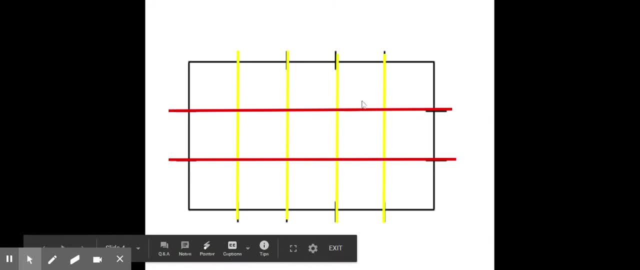 We have one, two, three, four, five columns. So to show that we would write three rows, five columns, And to get the total number of square units, we would count the total number of squares in the rectangle, which happens to be 15 square units. I can count that by skip counting. 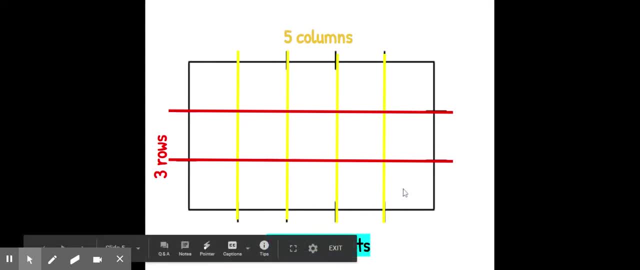 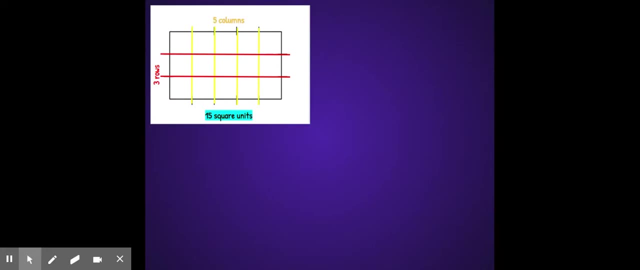 Five, 10,, 15.. Or I can count it by threes, Three, six, nine, 12,, 15.. But in second grade, remember, we are not counting One, two, three, four, five. Instead, we are skip counting. So if we want to represent that, 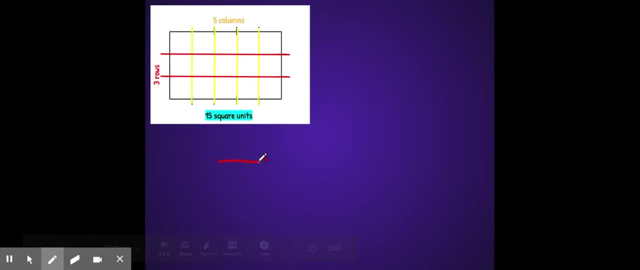 mathematically, we would show the number of rows, which is three rows- One, two, three- And we would write the number of columns on each of these lines: Five columns. so five plus five plus five equals 15.. Since you're on your way to third grade, I'll show you the multiplication form which you will be. 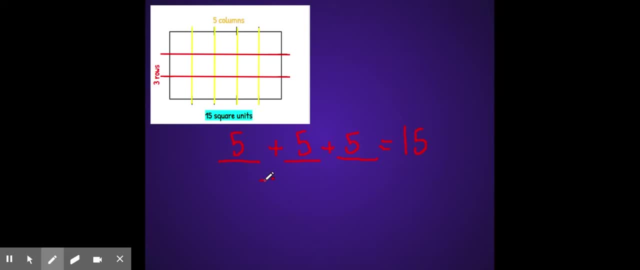 doing a lot of in third grade. So that would be three rows of five columns, which equals 15.. So that would be three rows of five columns, which equals 15.. So that would be three rows of five columns, which equals 15..